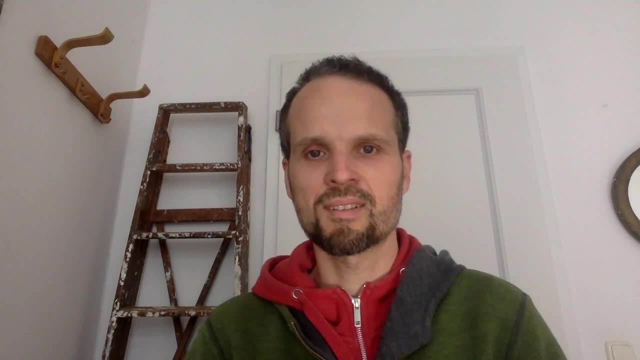 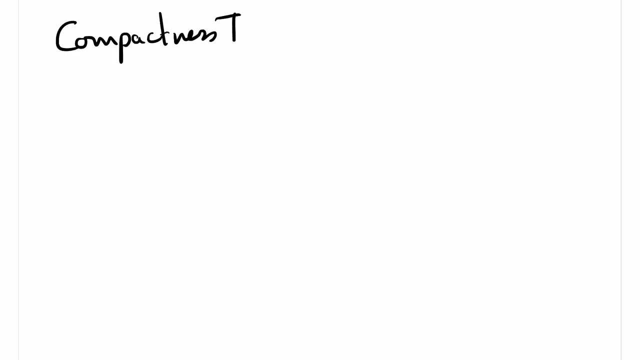 Hi. this video presents a proof of the compactness theorem of first-order logic based on the beautiful ultra-product construction. The compactness theorem states that if a first-order theory, that is, a set of first-order sentences, is unsatisfiable, that is, has no models. 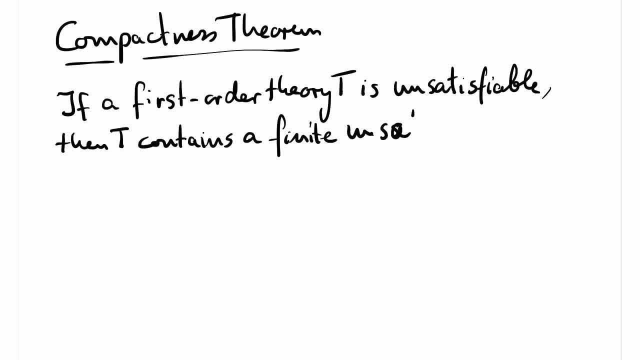 then it contains a finite, unsatisfiable subset. As I said, we use ultra-products to prove this theorem, which we of course need to introduce first. The compactness theorem is one of the most often used theorems of model theory. We will see. 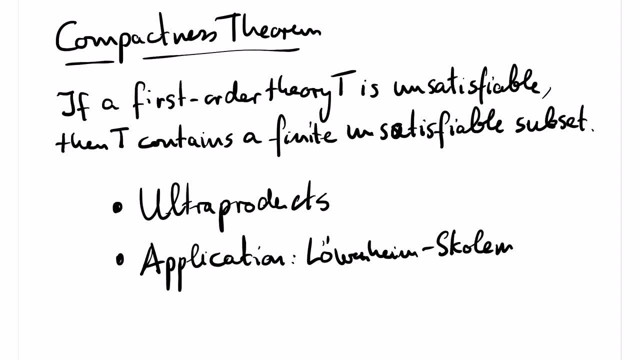 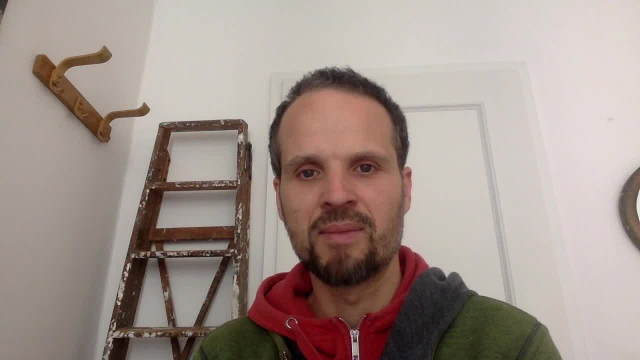 one application already in this video We use it to finish the proof of the Leuvenheim-Scholem theorem. One way of proving the compactness theorem is based on the completeness theorem of first-order logic. So this is a very proof-theoretic and syntactic approach. Here we take a different. 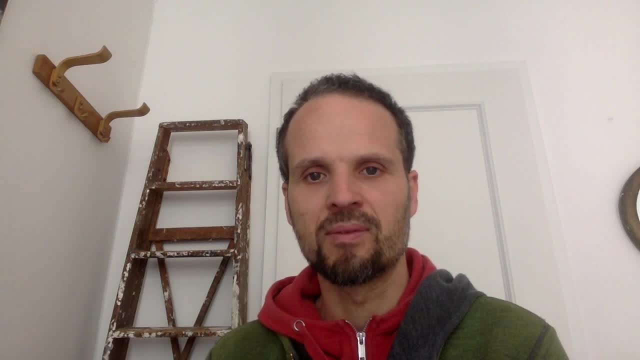 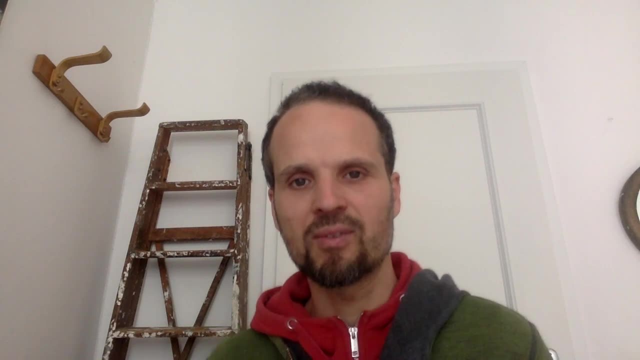 approach. We rather take the perspective of the contrapositive. Suppose you have a theory such that every finite subset of the theory has a model and we would like to construct a model of the entire theory. So it's really about constructing models here And ultra-products. 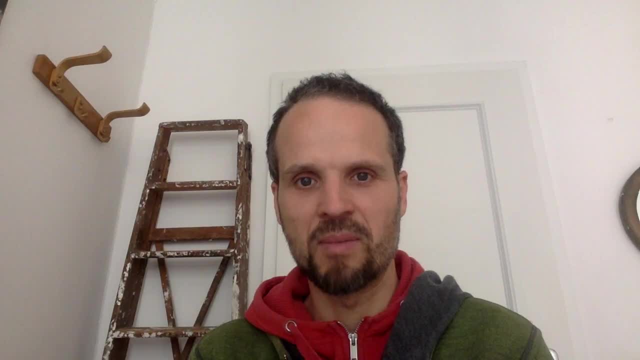 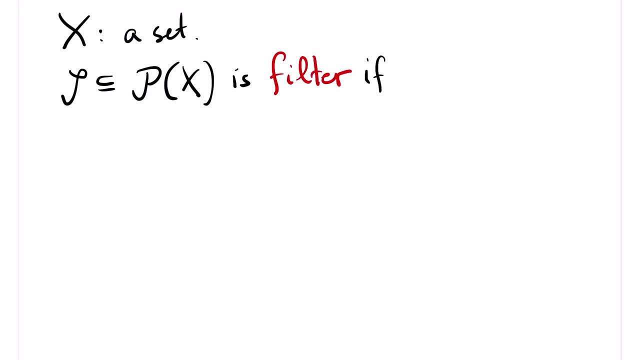 are a tool for doing this, So I will introduce them now. Let X be a set. A set S of subsets of X is called a filter if three conditions are satisfied. Before I give you the conditions, I will tell you what the intuition is. We imagine the elements of S. 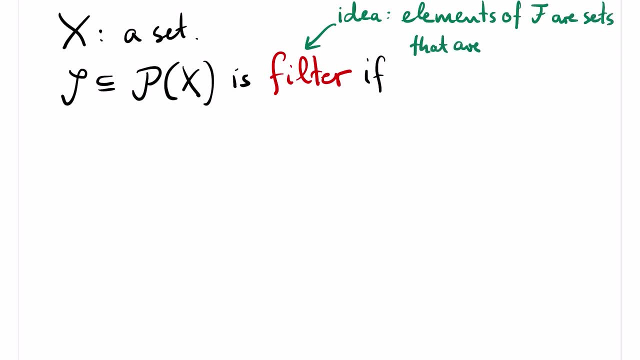 as very large. Actually, we imagine them as almost all of X. The first condition is that the empty set is not contained in S And X. the full set is in S. Well, the empty set is certainly not large and the full set certainly is large. So this matches. 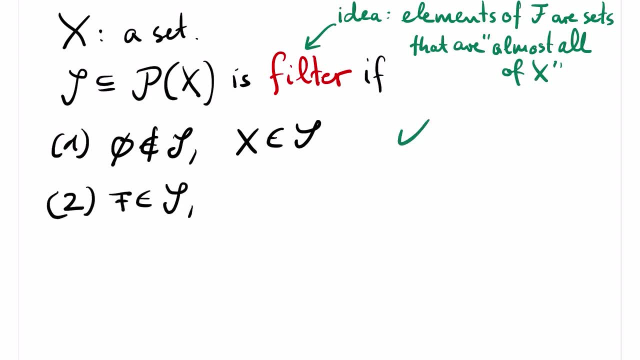 the intuition. The second condition is: if S is in S and F is contained in some larger subset G of X, then G is also in S. Again, this matches the intuition. If you add some elements to a large set, the resulting set is still large. The third condition is that if 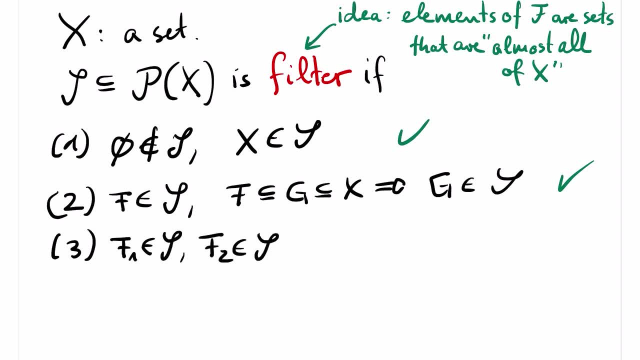 F1 is in S and F2 is in S, Then the intersection of F1 and F2 is in S. So it is important to imagine the elements of S as not just a large set but almost all of X. And then this again matches the intuition: if f1 and f2 are so large that they are almost 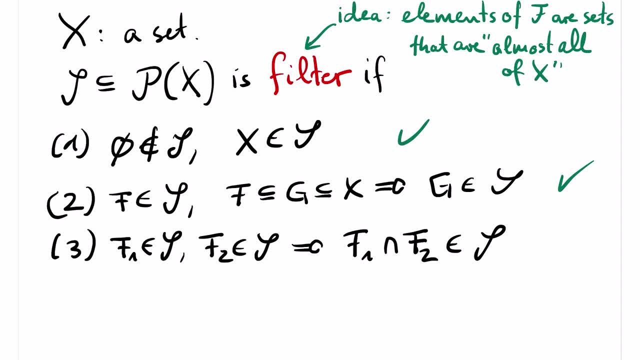 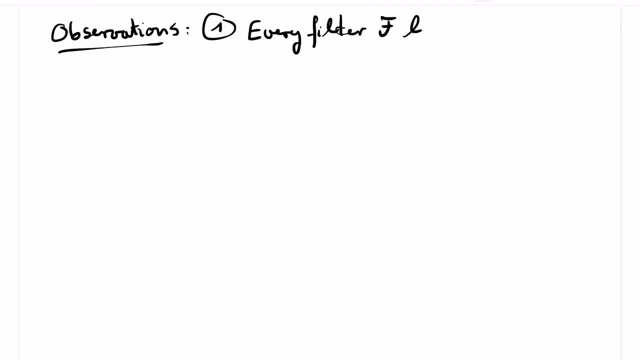 all of x, then their intersection is also almost all of x. Some observations about filters. Every filter f has the FIP, the finite intersection property, which states that if a1 up to an are sets in f, then their intersection is non-empty. 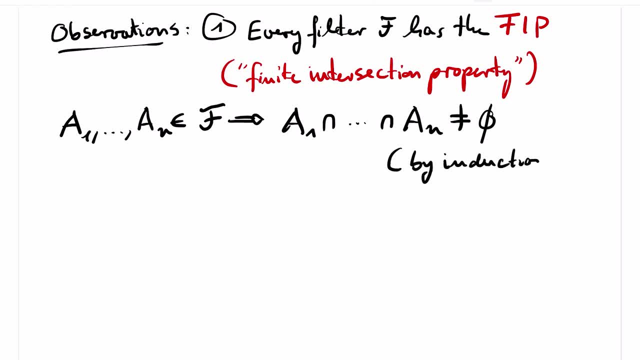 You can show by induction that the intersection is in f and the statement follows, since the empty set is not in f. Another observation is that every family s of subsets of x with the FIP is contained in a smallest filter that contains s. This filter is called the filter generated by s. 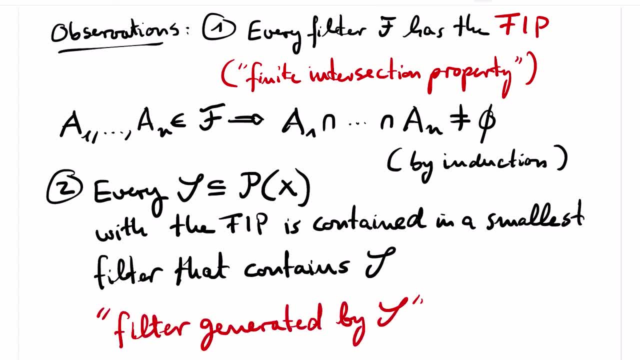 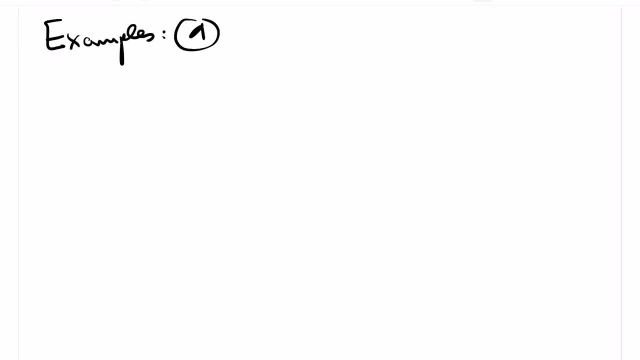 To see this, we first close s under finite intersections and then close it under finite intersections. The resulting family will be a filter contains s and is smallest. with these properties. I will give some examples of filters. For the first type of example, we fix 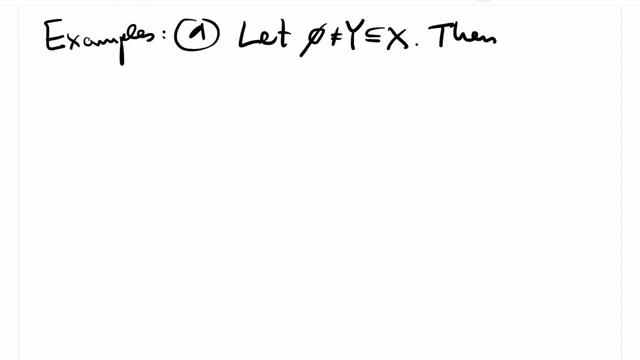 a non-empty subset y of x and include in our family f all sets that contain y, It's easy to check that f is a filter. Such filters are called principal. An example of a non-principal filter can be obtained from an infinite set x by including in our family f all subsets of x whose complement is finite. 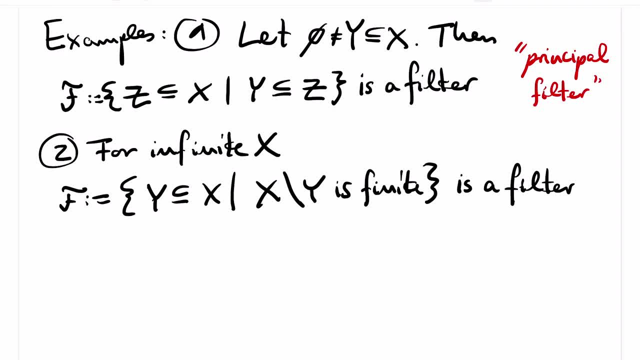 Again, it is easy to check that the three conditions for filters are satisfied. This is called the Frechet filter. on x A filter f is called an ultra-filter if f is maximal, That is, any filter that contains f must be equal to f. 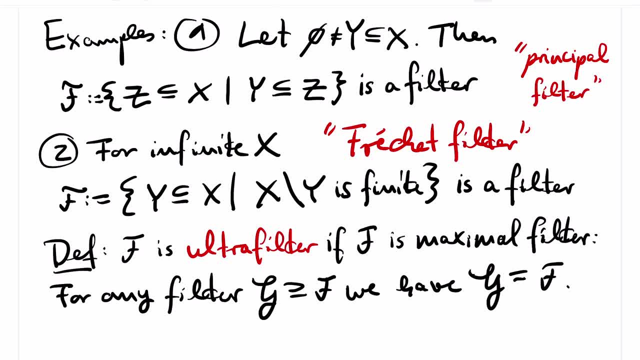 We cannot make f larger without losing the property to be a filter. A principal filter, for example, is an ultra-filter if it consists of all sets that contain one particular fixed element. The Frechet filter is not an ultra-filter. The principal ultra-filters are somehow boring, so it would be good to have some more examples. 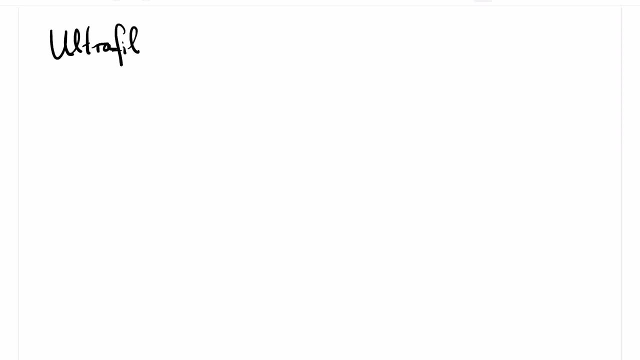 The following lemma shows that non-principle ultrafilters do exist. Our proof of the lemma uses the axiom of choice. ZF alone is not sufficient to prove the lemma. One can show that if ZF is consistent, there are models of ZF where the ultrafilter lemma does not hold. 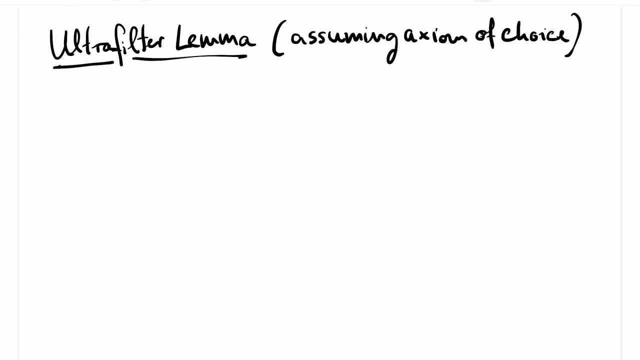 So we need to add something to ZF to prove the lemma, and the axiom of choice does the job. The lemma states that every filter F is contained in an ultrafilter. The proof is quite short. We consider the set of all filters on X that contain F. 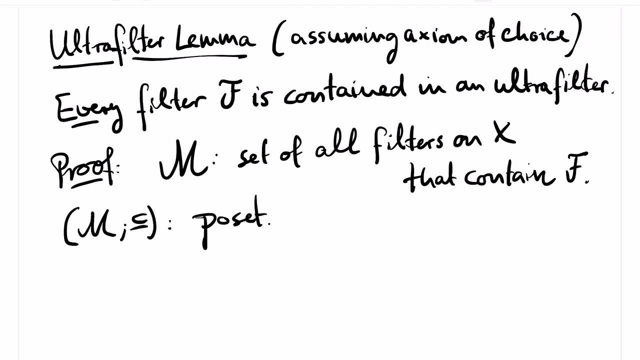 Then this set M forms a poset with respect to the inclusion relation. Note that the union of a chain in this poset. so this is just a sequence of elements that are increasing with respect to the inclusion relation, that the union of a chain is again a filter. 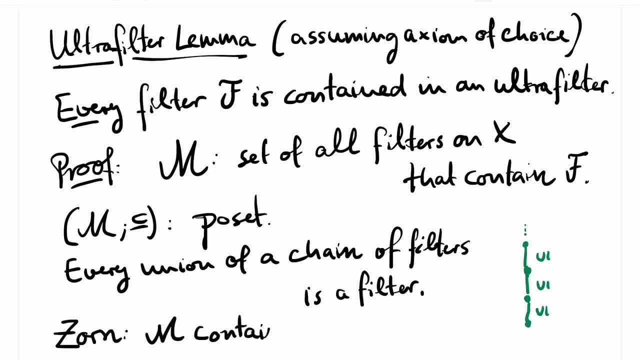 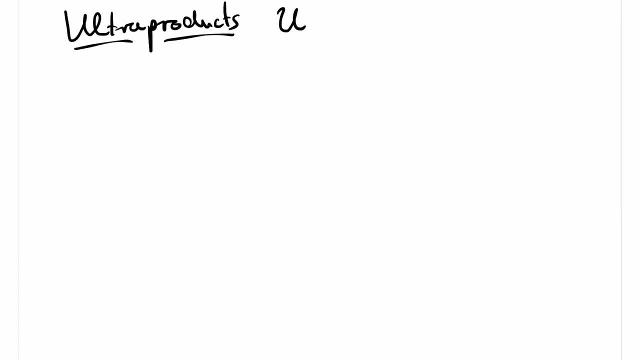 So Zorn's lemma, which is equivalent to the axiom of choice, implies that M is a filter, M contains a maxima filter. To define ultraproducts, we need an ultrafilter U on the set X and an infinite family of tau structures, MA, indexed by elements of X. 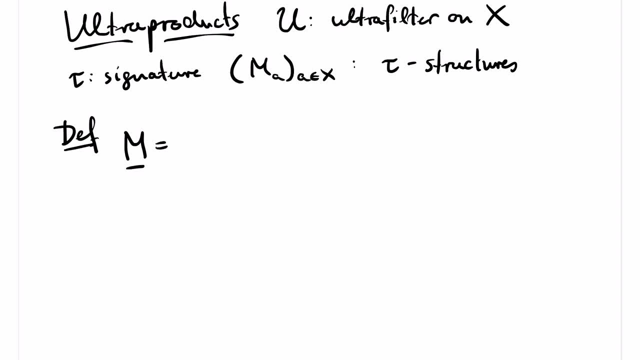 The idea is to define some sort of average structure that will have all the properties that hold in almost all of the factors MA. Our notation for ultraproducts M is that we write the product of the MI and then factor by the ultrafilter. 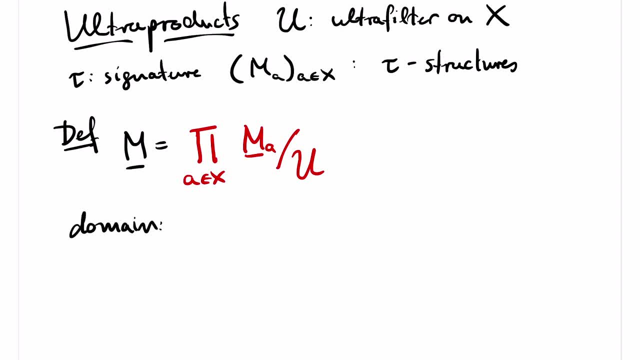 To define the structure M, I will first define the domain of M and then I define how the relations and functions of M look like. To define the domain of the ultraproduct M, we start with the set of all functions G from the index set X to the union of the MI. 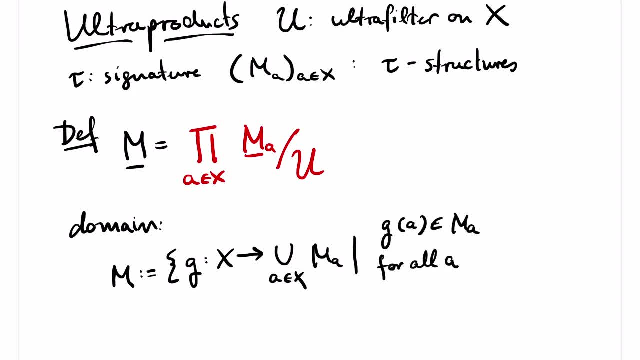 such that G maps an index A to an element of MA And then we factor this set by an equivalence relation that is obtained from the ultrafilter. We say that two functions are equivalent if the set of all indices where the two functions agree is in the ultrafilter. 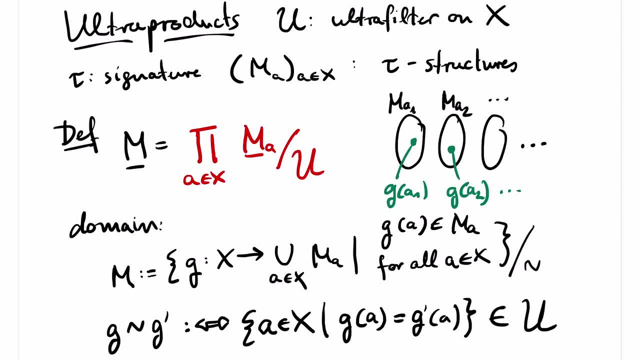 In other words, the two functions are almost always the same. The domain of our ultraproduct contains the equivalence function, so we can define its classes with respect to this equivalence relation. In other words, we start from the usual product and then identify elements of the product. 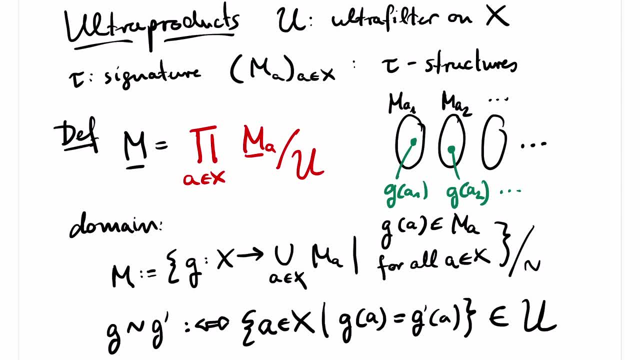 that are equal on almost all coordinates. With the idea that M should be an average structure over all the MI, the definition of how the functions and relations of M look like is clear. We start slowly with constant symbols in tau, even though this is a simple equation. 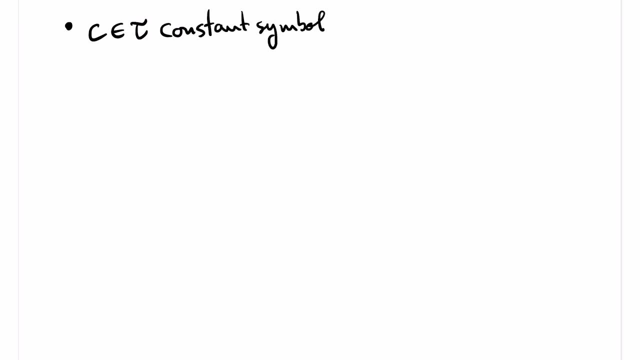 but it is a special case of function symbols. So if C is a constant symbol in tau, this constant symbol denotes in the ultraproduct the equivalence class of the function that maps an index A to the element of MA. that is denoted by the constant in MA. 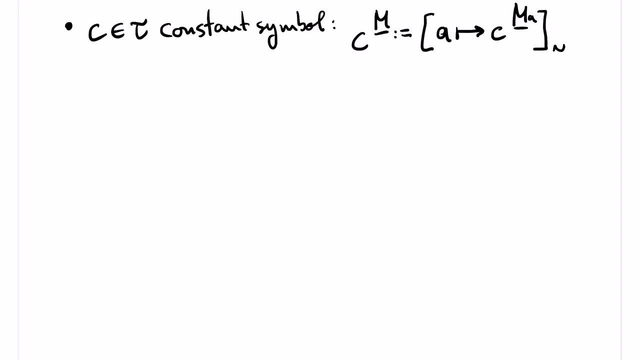 My notation for equivalence classes is that I put brackets around a representative of the class And I put the equivalence class of A around the class And I put the equivalence classes around a representative of the class equivalence relation as a subscript. later this subscript can also be omitted if it is clear from. 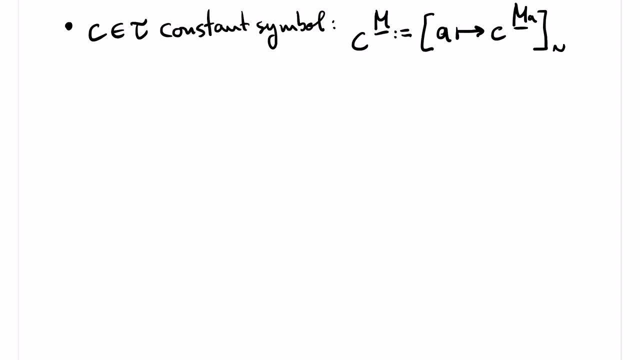 the context, which equivalence relation i mean. before we define how functions look like in m, we define how the relations of the ultra product look like. then it's slightly easier and gives the idea for functions as well. suppose we have a relation symbol r of ret k in our signature. 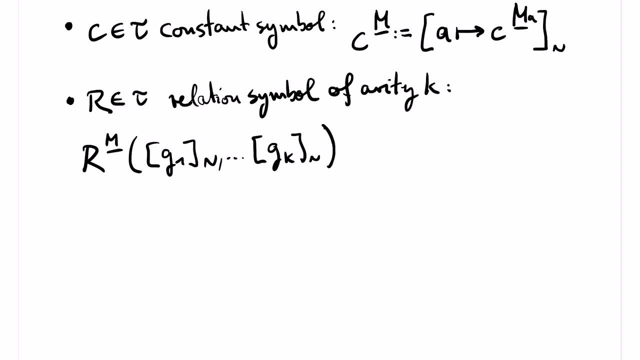 the idea is to put a tuple into the relation for r in the ultra product if in almost all of the factors the relation holds on that tuple. formally we look at the set of all indices a such that the relation holds in the eighth factor. this set of indices should be contained in the 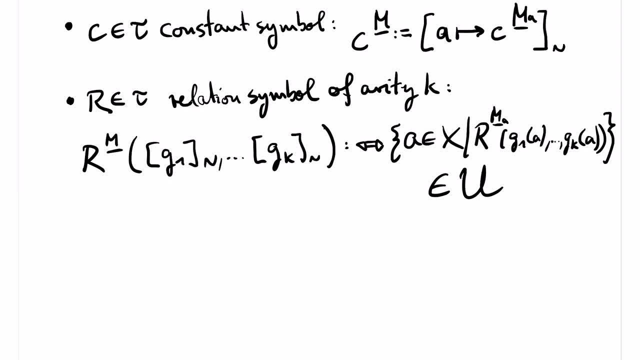 ultra filter. so the ultra filter codes what it means that the relation holds in almost all of the factors. you With the case of relation symbols in mind, function symbols can be treated in the same way. we simply apply the definition for relations to the graph of the function. if the function 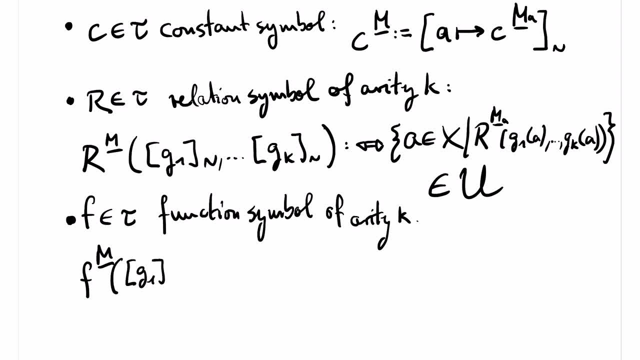 symbol has r ret k, then the graph of the function symbol is the relation of r ret k plus one that is defined by the atomic formula. f, applied to some elements, equals some other element. such an atomic formula holds in the ultra product if, and only if, the set of all indices a, such that the formula holds in the eighth factor, is in the ultra filter. so again, the intuition being that the atomic formula is true in the ultra product if, and only if, it holds in almost all of the factors. 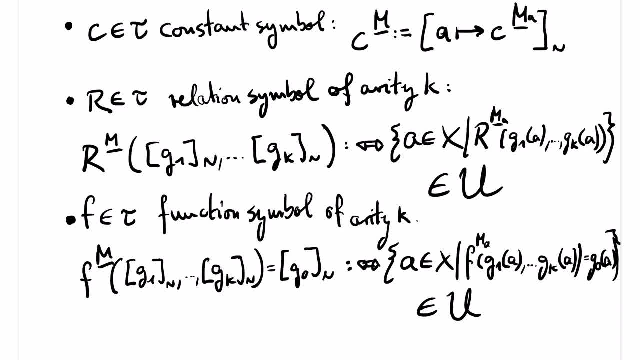 We still have to check that this is well defined. the definition should not depend on the choice of the representatives from the equivalence classes. this is straight forward but somewhat tedious, so I leave for now this as an exercise. Actually, the definition makes perfect sense also for filters. We don't 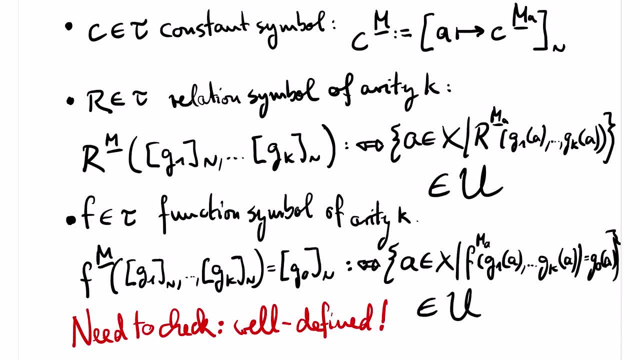 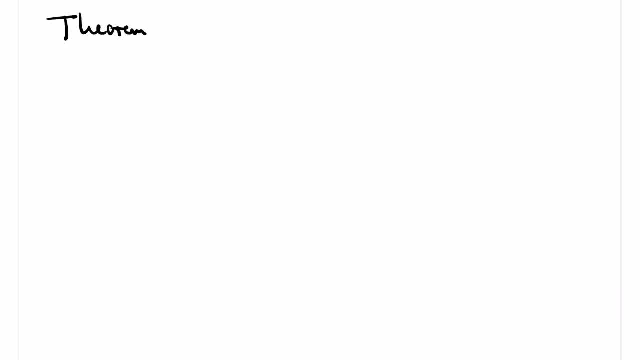 need ultra filters. In this case, the resulting structure is called a reduced product, not an ultra product. What can we say about ultra products? The first thing that we have to prove is the theorem of WASH. It clarifies which first-order sentences hold in the ultra product. 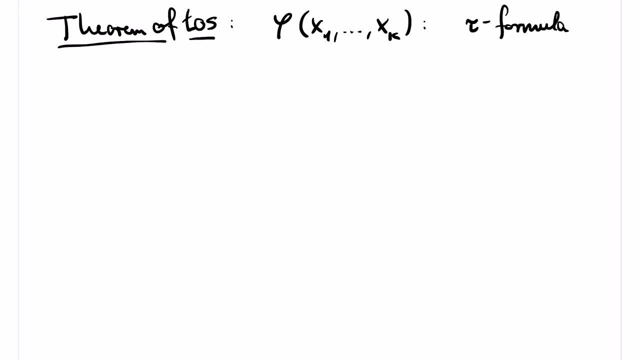 In fact we prove a statement about formulas, not just sentences. Let phi be a tau formula with three variables: x1 up to xk. We pick also k elements of the ultra product. We would like to know whether the ultra product satisfies phi applied to these elements. The theorem. 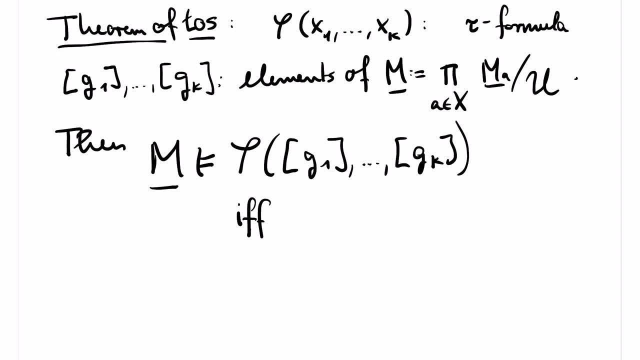 of WASH tells you that it suffices to check the formulas in the factors. If it holds in almost all of the factors, then it also holds in the ultra product and vice versa. This can be shown by analysis. It is tempting to skip such proofs, but actually I decided not to skip it because it shows. 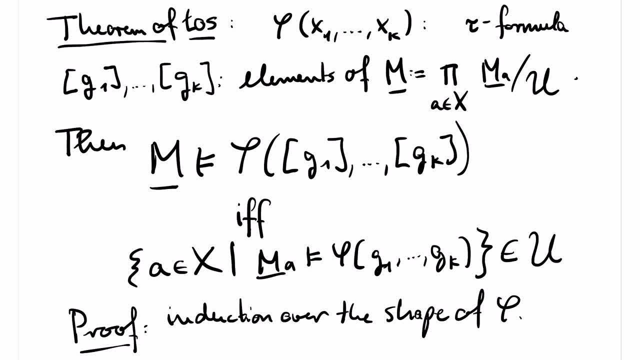 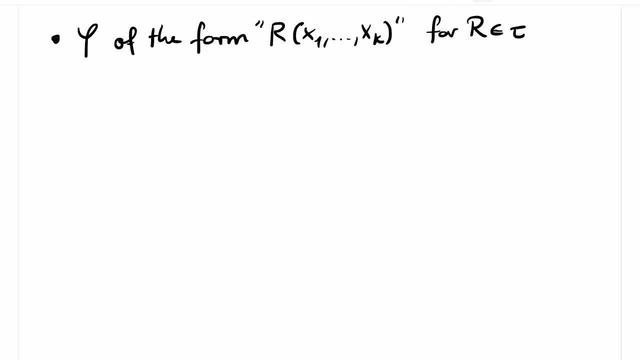 how nicely all the concepts play together. We start with atomic tau formulas. For simplicity, we only do it with atomic formulas built from a relation R, say of R-U-T-K. The statement is then immediate from the definition of the ultra product. Next we look at formulas built 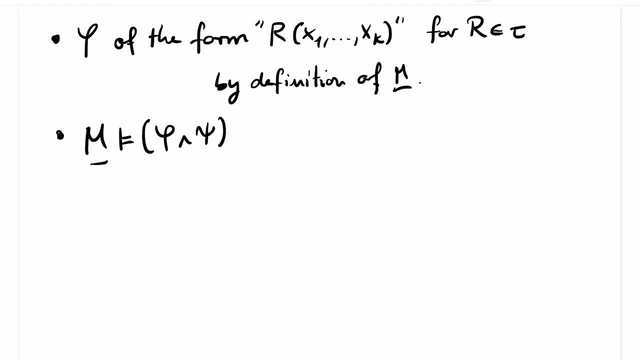 from smaller formulas phi and psi With conjunction m models phi and psi at the selected elements if, and only if, m models phi and m models psi. Since phi and psi are smaller formulas, the inductive assumption gives us that we may evaluate the formulas in the factors. 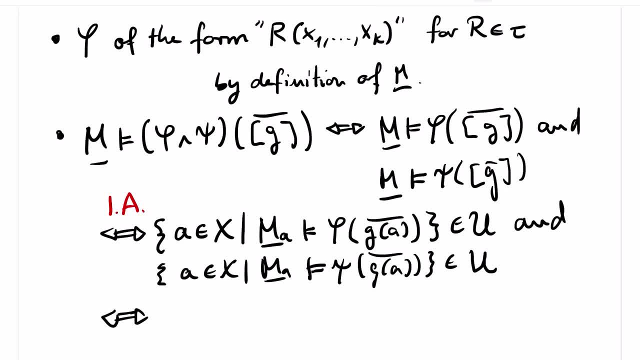 And now we use the fact that the ultra filter is closed, undertaking finite intersections. The set of indices where phi holds is in the ultra filter and the set of indices where psi holds is in the ultra filter if, and only if, the set of indices where phi and psi holds. 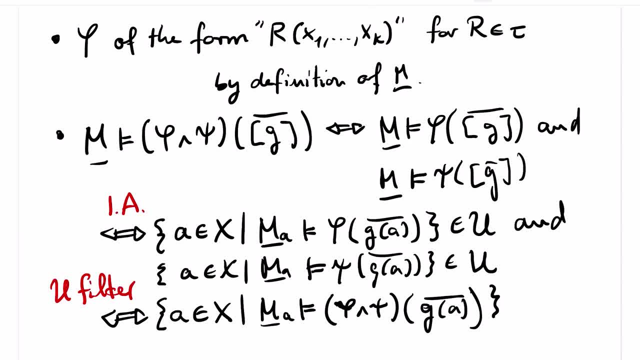 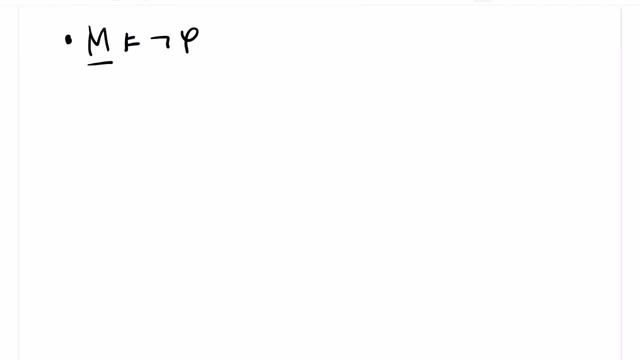 is in the ultra filter, And this is what we wanted to show. Next, we consider a formula that is built from a smaller formula, phi, by negation. Our ultra product m satisfies not phi at the chosen elements, if, and only if, m does not satisfy. 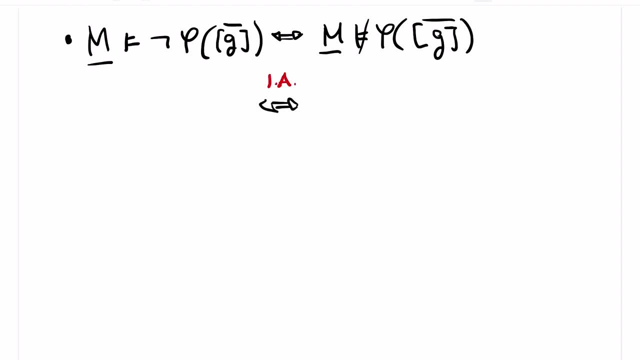 phi. Next, the set of indices where phi and psi do not satisfy phi, which by inductive assumption holds if and only if, the set of indices A, such that m A satisfies phi, is not in the ultra filter. And now we use for the first time that U is an ultra filter and not just a filter, The 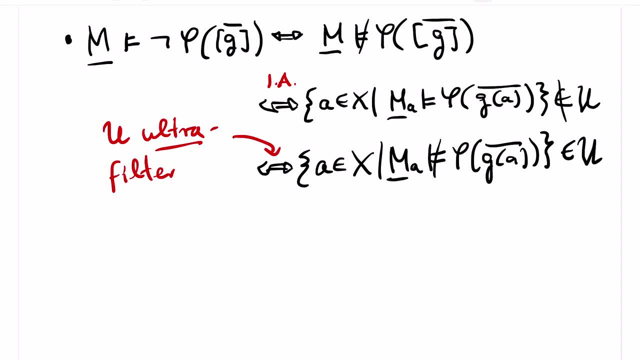 maximality of U implies that in this case, the complement of the set of indices must the resulting set under intersections and supersets and would obtain a larger filter, which is impossible by the maximality of u. So we have that the set of indices a, such that m a satisfies, not phi, is in the ultra filter, which is what 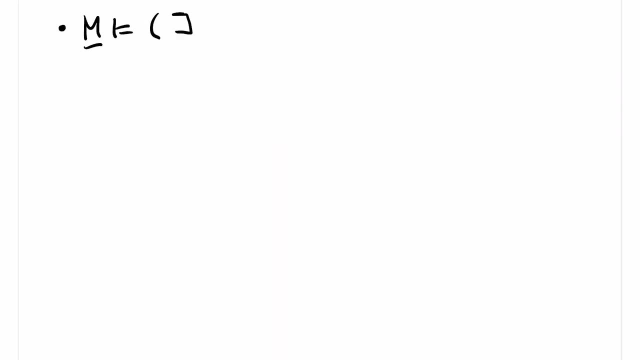 we wanted to prove. Finally, we have to look at the case that a formula is built from a smaller formula, phi, by existential quantification. Our ultra product m satisfies such a formula at the chosen points, if, and only if, there exists a witness for the existentially quantified variable in the ultra product. 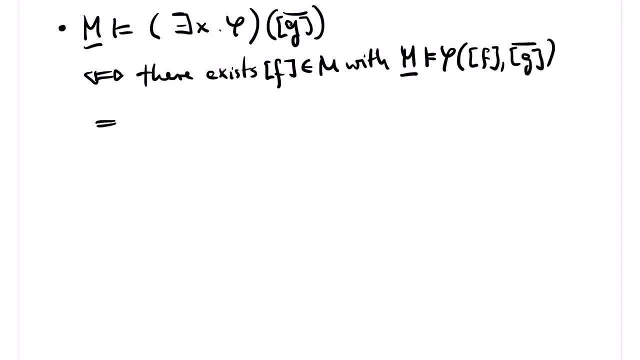 such that phi holds for this witness. With the inductive assumption, we can again translate this into a statement about almost all of the factors. I claim that this statement holds if, and only if, the set of indices a, such that m a satisfies, exists. x, phi is in the ultra filter. The forward direction is clear. 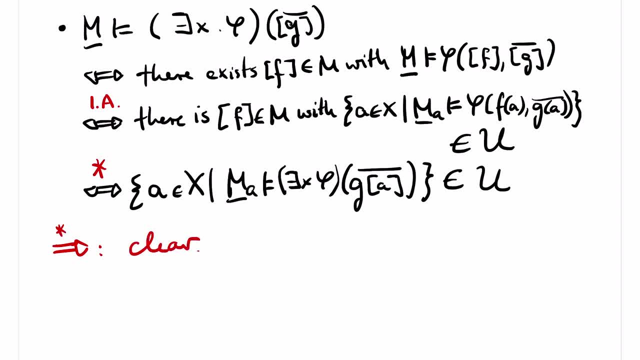 since the witness applied to index a shows the statement for m a. For the converse, suppose that a is an index such that m a satisfies: exists x, phi. Let h a be a witness for the existence of such an x. We now define a representative f of. 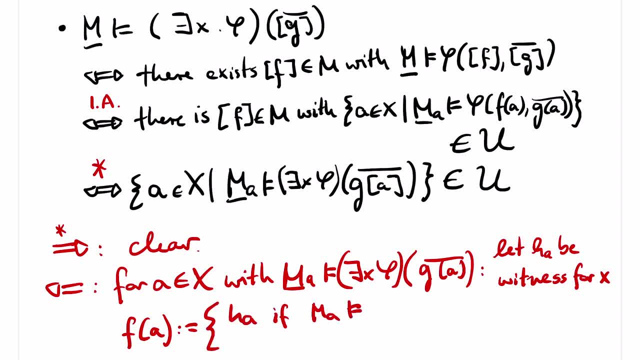 the desired witness in m as follows: If a is such that m? a satisfies exists, x, phi, then f of a is defined to be h? a. Otherwise f of a is set to an arbitrary element of m? a. It's now not difficult to verify that the equivalence class of f 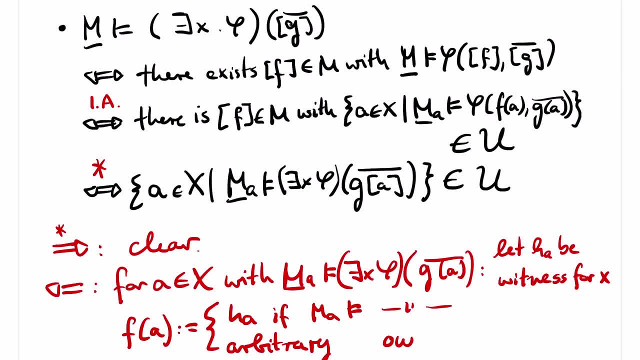 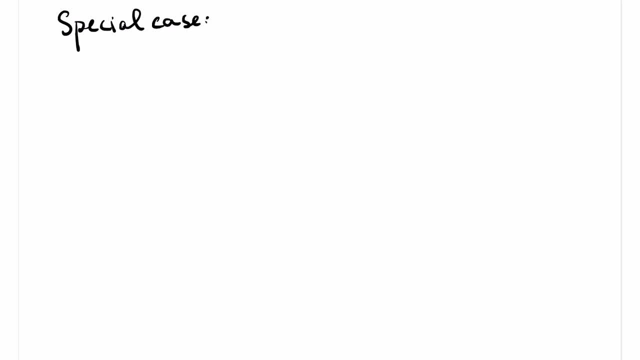 satisfies phi in m. And this concludes the proof of Walsh's theorem. Ultra powers are a special case of ultra products where all factors are the same structure, a. We use the following notation: a to the x is the usual power of a, where x is an index set for the factors of the power. The notation for: 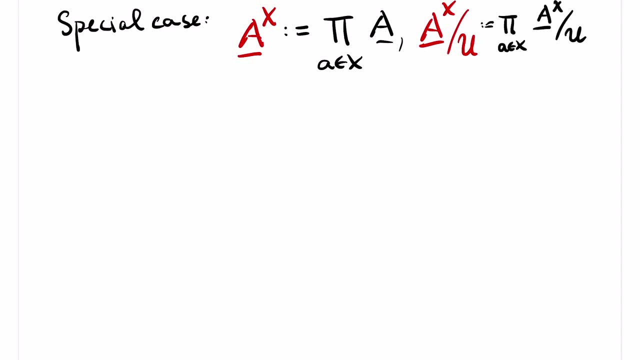 ultra powers is analogous. We write a to the x factored by a for the respective ultra product, where all the factors are a. A corollary of Walsh's theorem is that the first-order theory of an ultra power of a structure, a, equals the first-order theory. 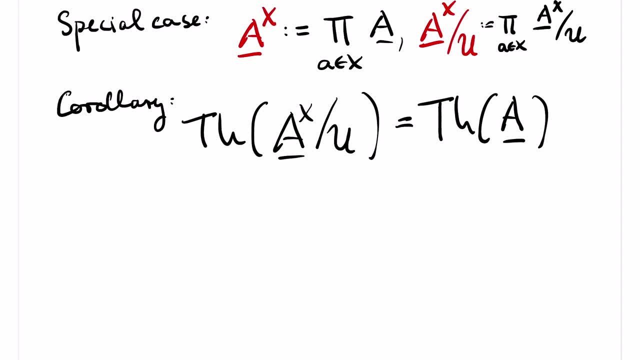 of a. We just apply it to sentences instead of formulas, and to ultra powers instead of ultra products. Every first-order sentence that holds in a holds in all factors of the power and therefore holds in the ultra power as well. This statement is trivial if the chosen ultra filter is principal. However, if we have a, 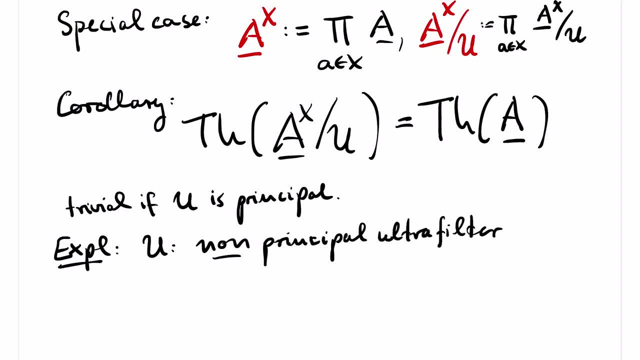 non-principal ultra filter. the statement is interesting. For example, consider a non-principal ultra filter on omega And now consider the ultra power of the structure, which is the natural numbers with addition and multiplication. with respect to this ultra filter, I claim that the 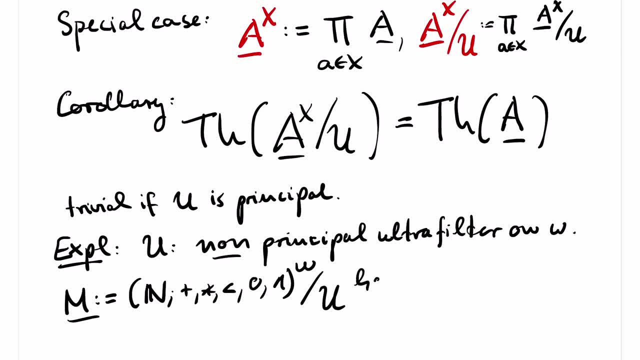 resulting structure has infinitely large elements, by which I mean elements u that are larger than every integer. Note that each fixed natural number, n, can be expressed using a term built from and addition, so we can express in first-order logic that u is larger than n. 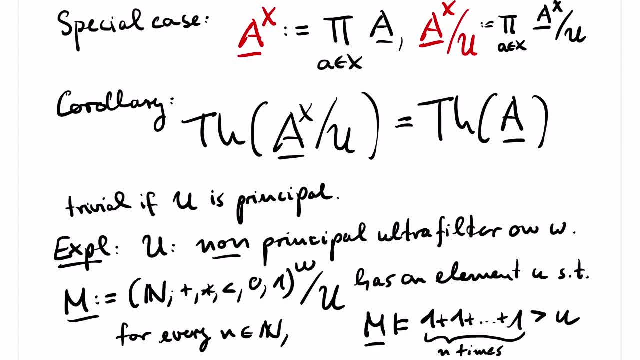 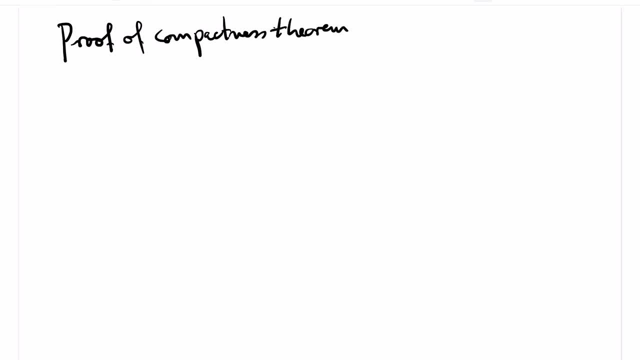 The example shows that ultra products are a powerful tool to construct interesting models of first-order theories. We are now ready for our super short proof of the compactness theorem. Let T be a first-order theory, such that every finite subset S has a perfect compactness value and the effect. 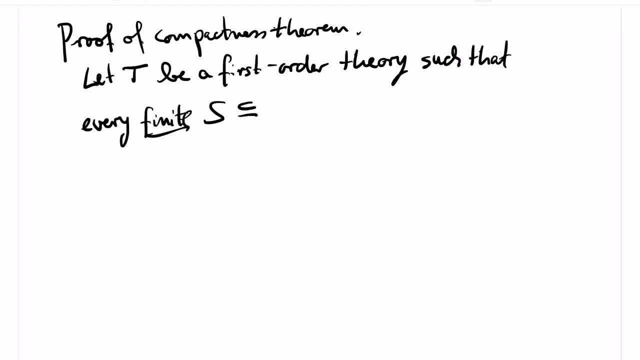 of a complex number of products can be reduced to a single magnitude. This implies that each s of t has a model, ms. We have to construct a model of t. Let x be the set of all finite subsets of t. For any first-order sentence, phi in t, we define x sub phi as the set of. 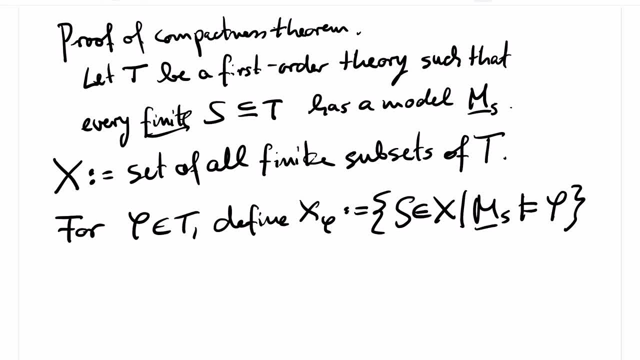 all finite subsets s of t, such that ms satisfies phi. We first prove that the family of all x phi for phi in t has the FIP, the finite intersection property. This is actually easy If phi1,, phi2, and so on until phi n are sentences. 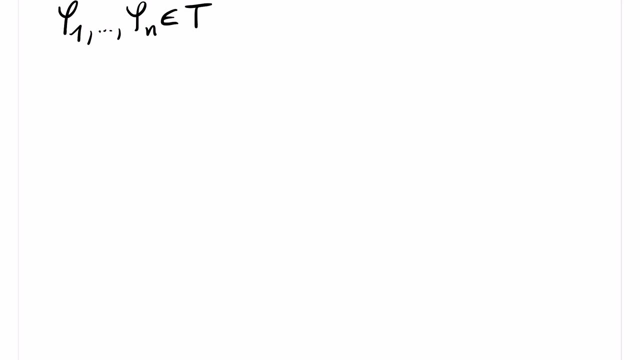 in t, we have to show that the finite intersection of x, phi1,, x, phi2, and so on is non-empty. Let s be the set that consists of exactly phi1 up to phi n. Let s be the set that consists of exactly phi1 up to phi n. Let s be the set that consists of exactly phi1 up to phi n. 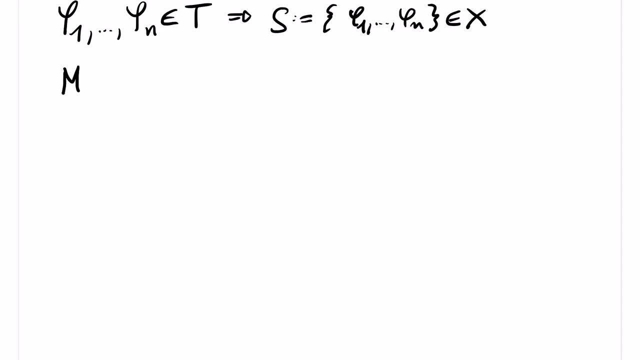 This is an element of x. Certainly ms satisfies phi i for every i. So s is contained in x phi i for every i, and hence in the intersection of all the x phi i, showing that this intersection is non-empty. This concludes the proof of the finite intersection property. 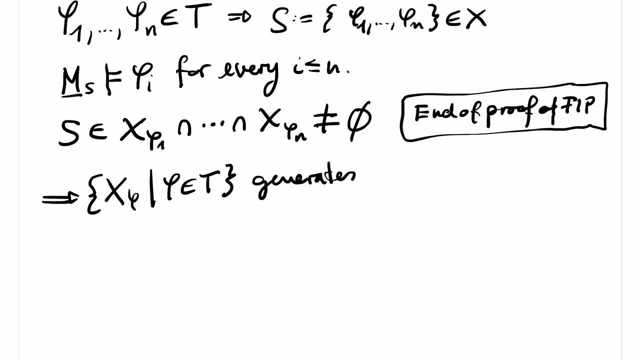 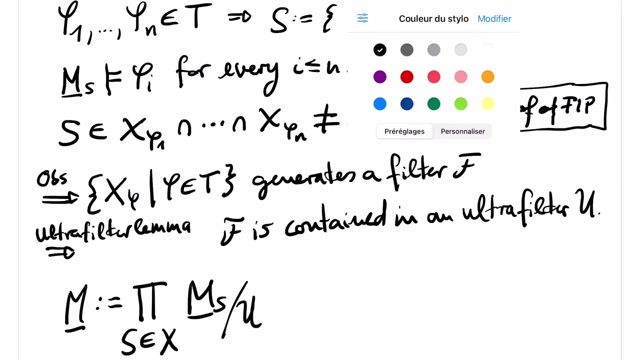 From the beginning of the video we know that every family with the FIP generates a finite intersection factors and that every parent with the FIP generates a set of gigabytes. When we first make dirty FIP heading- which we'll discuss later- we note that if alpha is the infinite intersection, 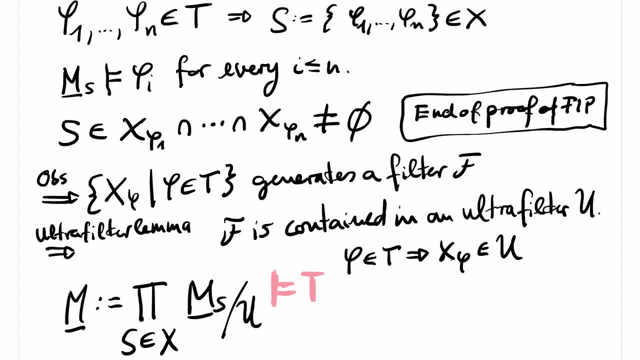 in t By the construction of u. the set x, phi is contained in the ultrafilter. u x phi equals the set of all elements of x, such that ms satisfies phi. So if this set is in u, then Walsh's theorem implies that m satisfies phi. So indeed m satisfies all sentences in. 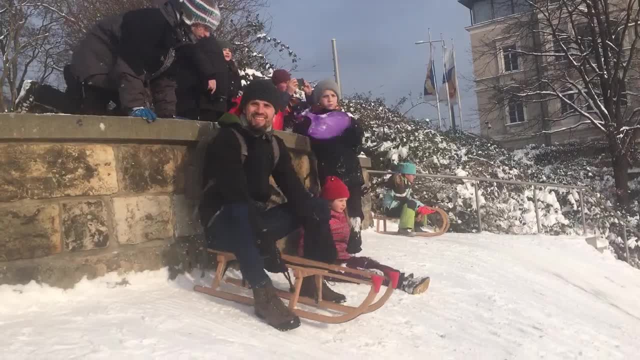 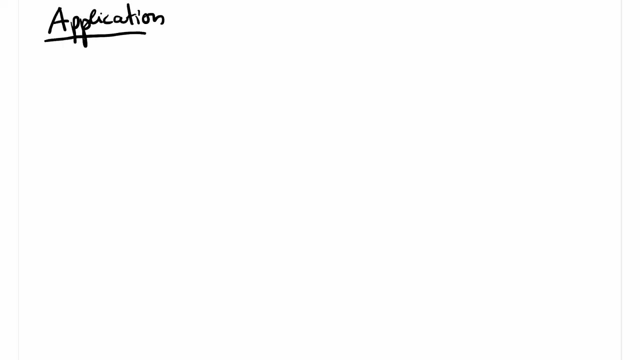 t. End of proof. We now use the compactness theorem to prove the Leuvenheim-Skolem theorem. Remember that the Leuvenheim-Skolem theorem states that if a first-order theory, t, has an infinite model, then it has models of all infinite cardinalities. This theorem has two parts. 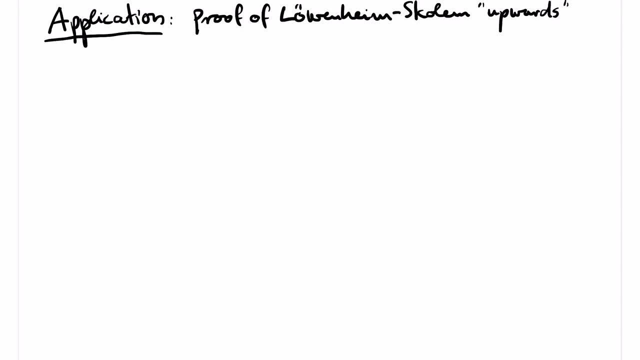 Leuvenheim-Skolem upwards and Leuvenheim-Skolem downwards, which we have already proved For up. we need to prove that if t has an infinite model a, then we can construct a larger model of t. So it suffices to prove that if a is an infinite tau structure and kappa is a cardinal, which is 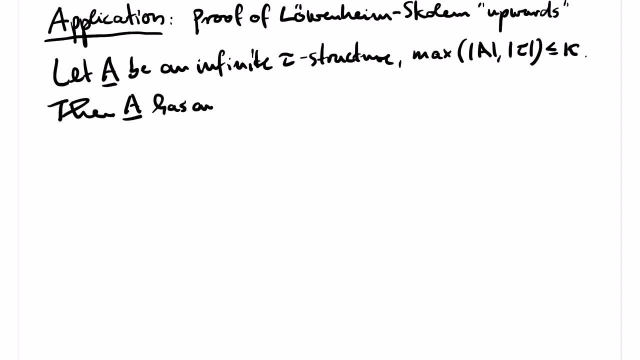 larger than the cardinality of a, then a has an elementary extension of cardinality, kappa. If our signature is uncountable, I also need that kappa is larger than the cardinality of the signature. In the first step we construct an elementary extension a' of cardinality, at least kappa.